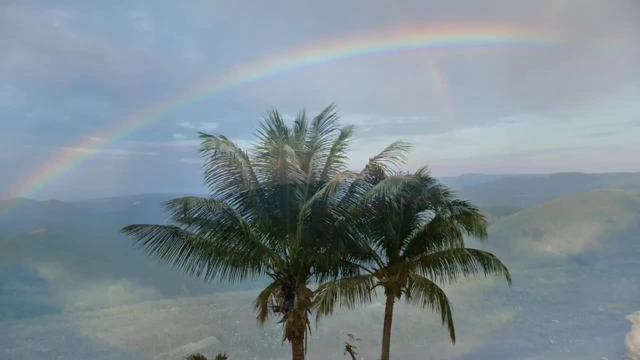 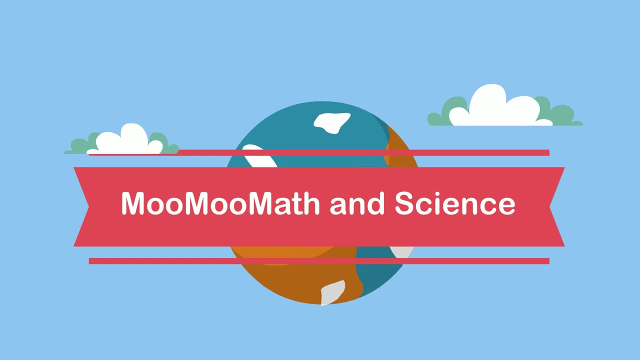 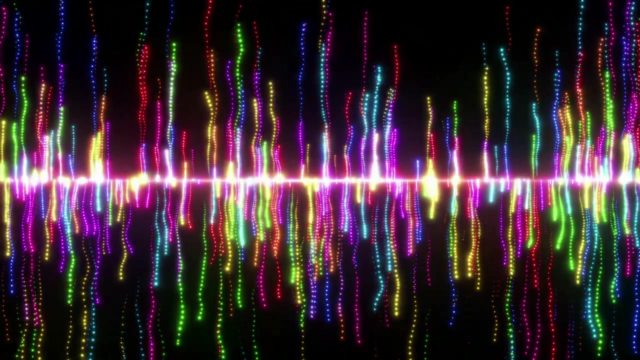 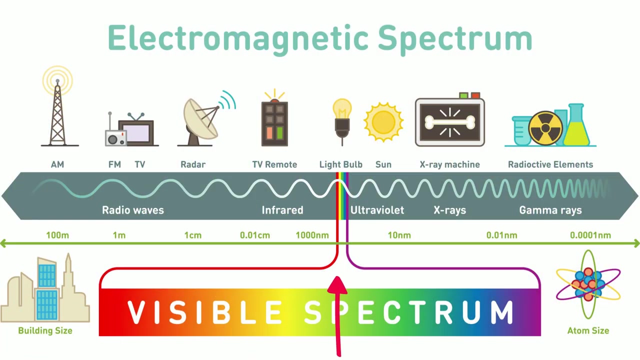 Almost everyone loves a rainbow. Rainbows are an example of visible light. Welcome to MooMooMath and Science in Visible Light. When you see a rainbow or other colors, you are viewing visible light. Visible light is the narrow range of wavelengths and frequencies found within the electromagnetic spectrum. It is found between: 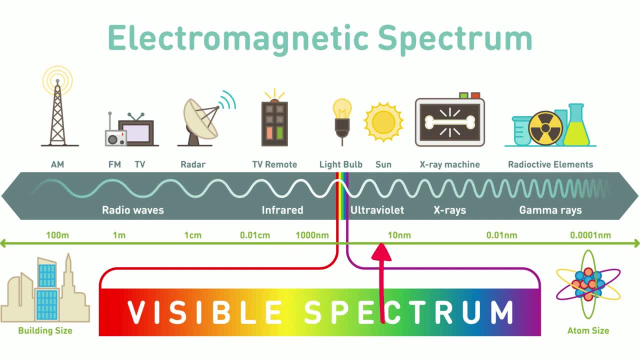 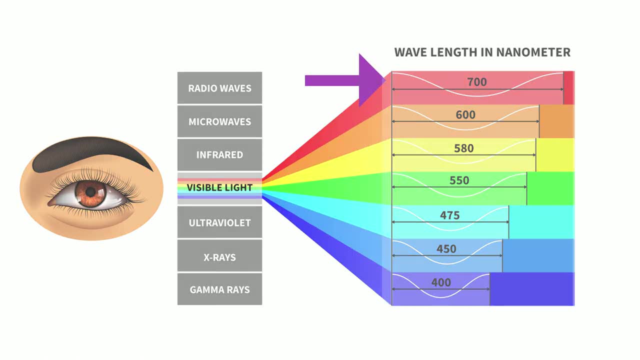 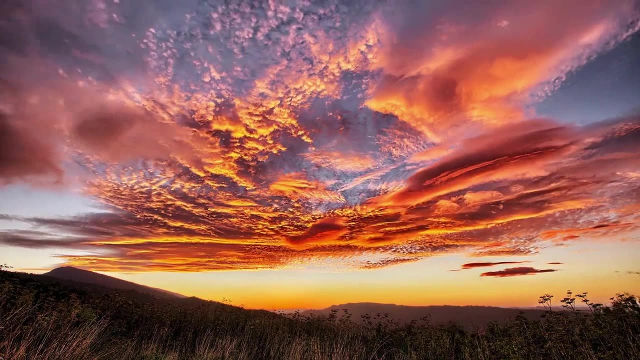 infrared waves and ultraviolet waves. Visible light has wavelengths of around 400 and 700 nanometers. When the sun rises and sunlight brightens the day, you are seeing white light. White light is the visible light of all wavelengths in the sky- Light from light bulbs. 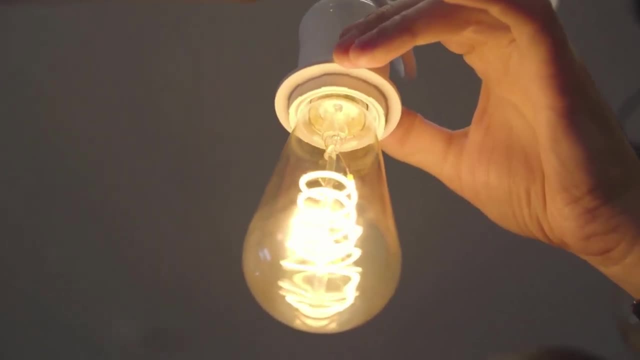 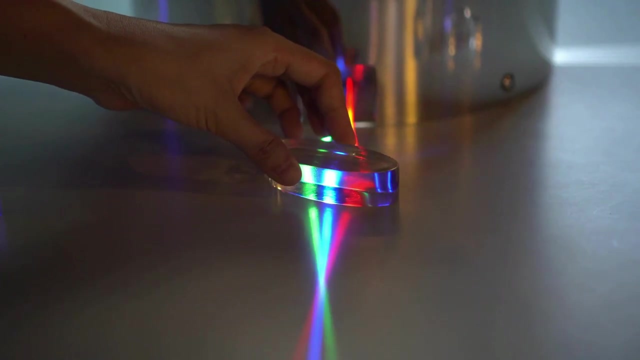 is also made up of white light. White light is made up of different wavelengths which result in Jacuzzi light. It is different wavelengths of light where the rays of light differences different colors. If white light passes through a prism, you can see these different colors. 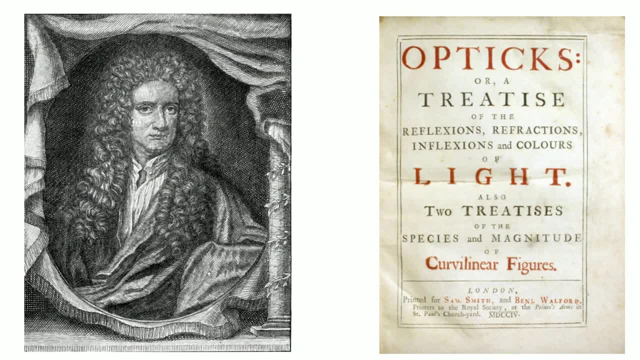 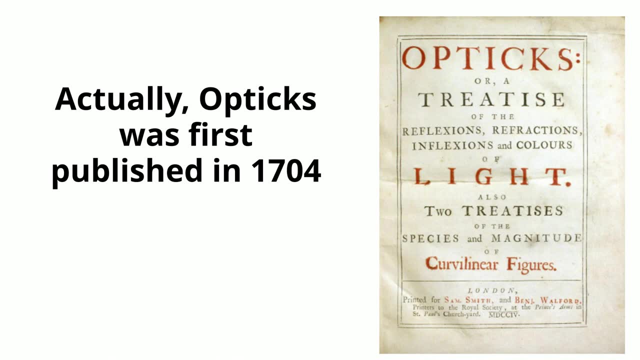 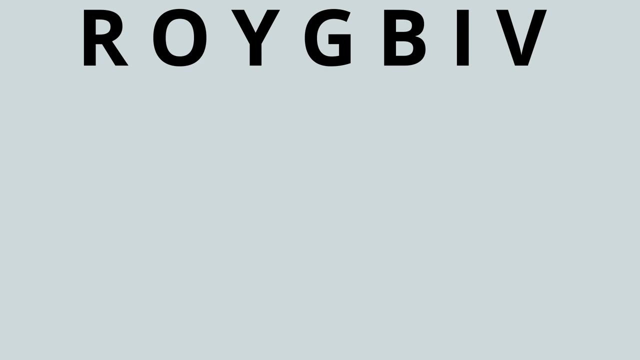 Interesting science fact. Sir Isaac Newton described how white light is made up of different colors in 1671 in his book Optics. An easy way to remember the colors of visible light is to use the name ROYGBIV, which stands for Red, Orange, Yellow, Green, Blue, Indigo. 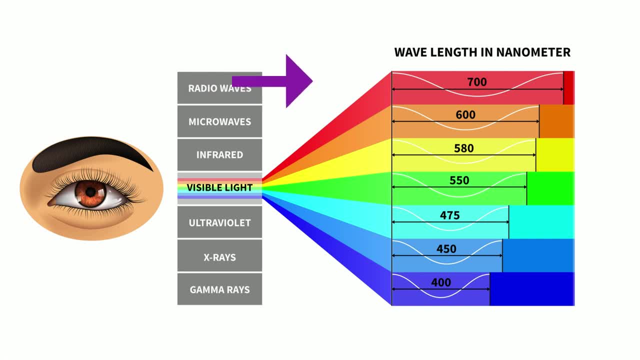 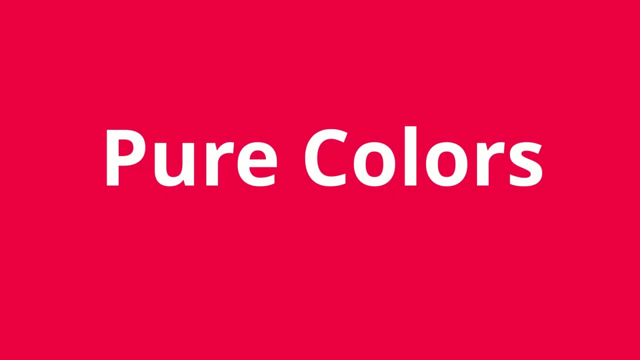 Violet Red light is found at the lower end of the visible spectrum. It has a longer wavelength of about 740 nm. Light in the middle of the spectrum is seen as green, and light at the upper end of the spectrum is green, Which has a wavelength of around 380 nm. is seen as violet Colors containing only one. 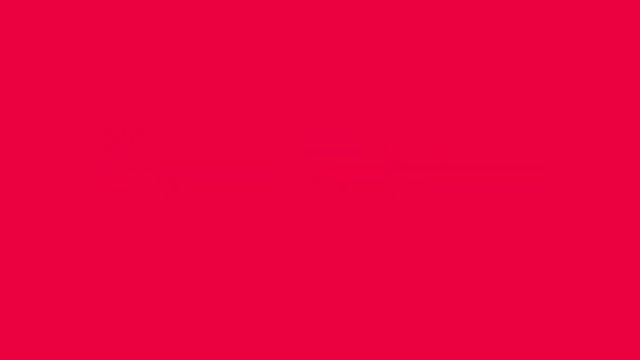 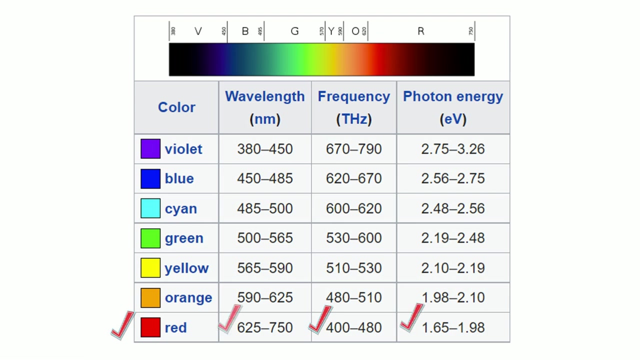 wavelength are also called pure colors, and they are red, green and blue. All other colors that we perceive are mixtures of these colors. Red light has the lowest frequency and photon energy, along with the longest wavelength, and violet has the highest frequency and photon energy, along with the shortest wavelength. 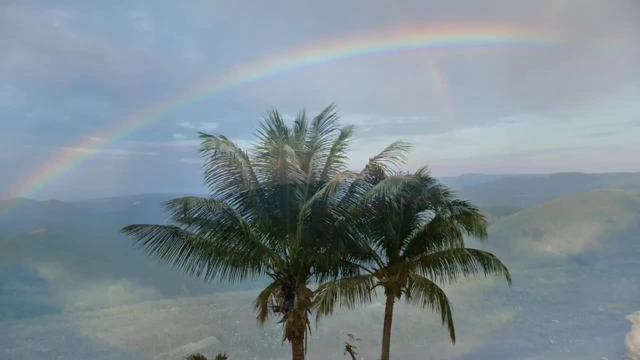 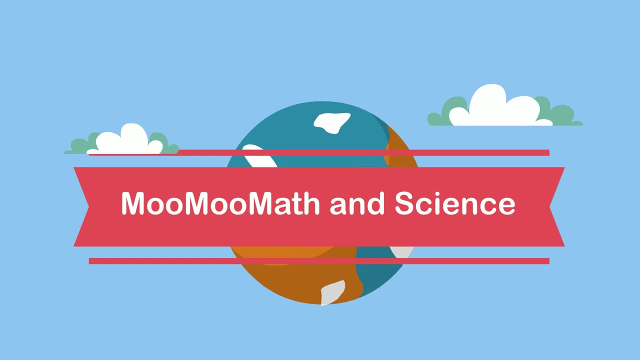 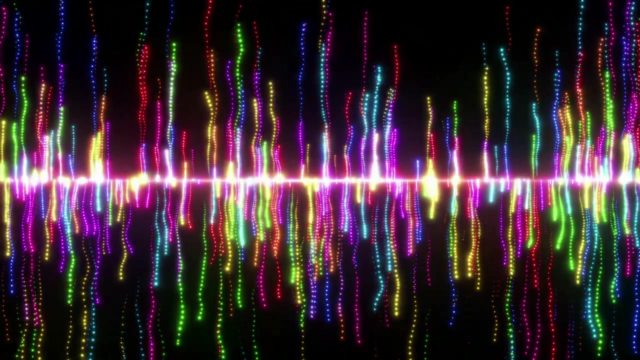 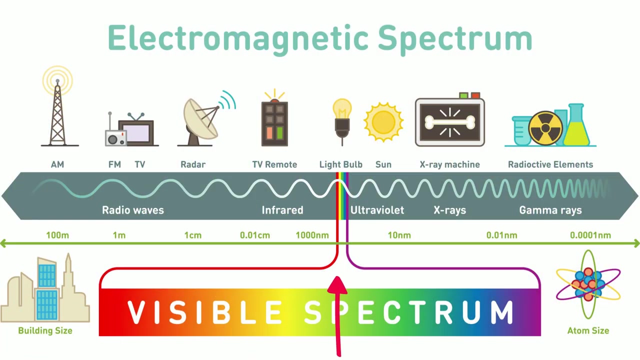 Almost everyone loves a rainbow. Rainbows are an example of visible light. Welcome to MooMooMath and Science in Visible Light. When you see a rainbow or other colors, you are viewing visible light. Visible light is the narrow range of wavelengths and frequencies found within the electromagnetic spectrum. It is found between: 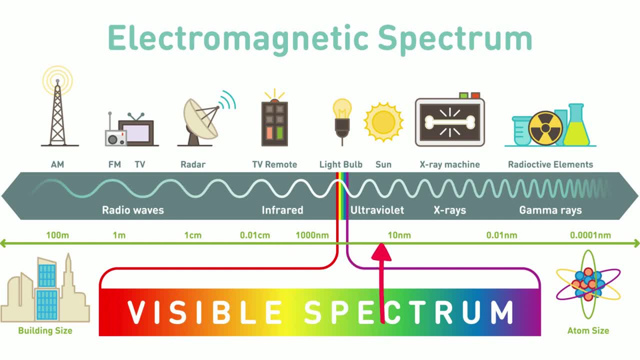 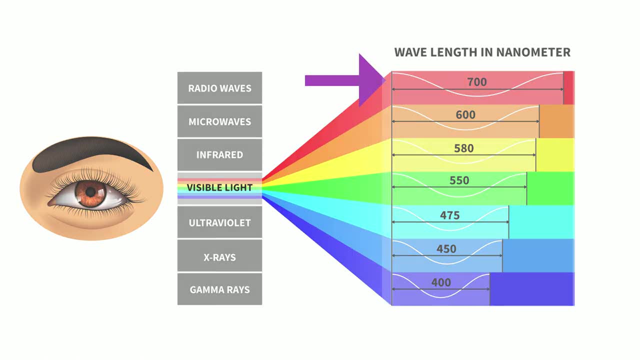 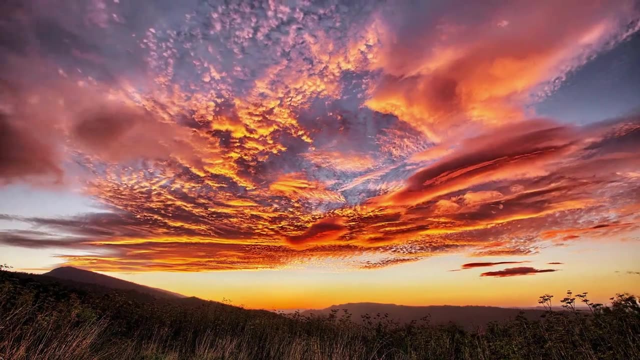 infrared and ultraviolet waves. Visible light has wavelengths of around 400 and 700 nanometers. When the sun rises and sunlight brightens the day, you are seeing white light. White light is the visible light of all wavelengths combined Light from light bulbs is also made up of white. 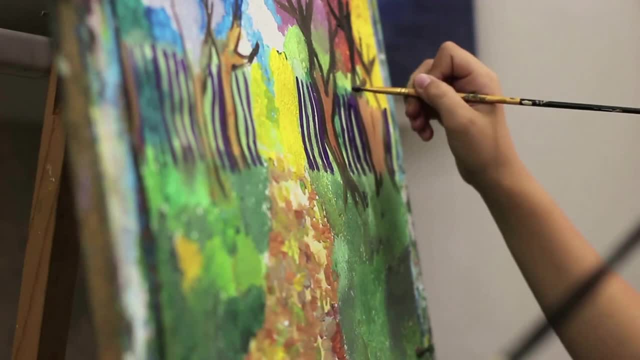 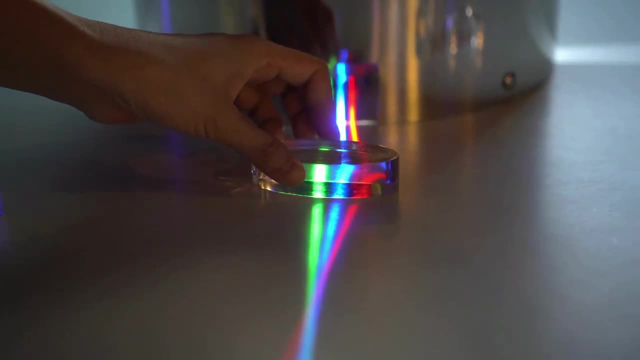 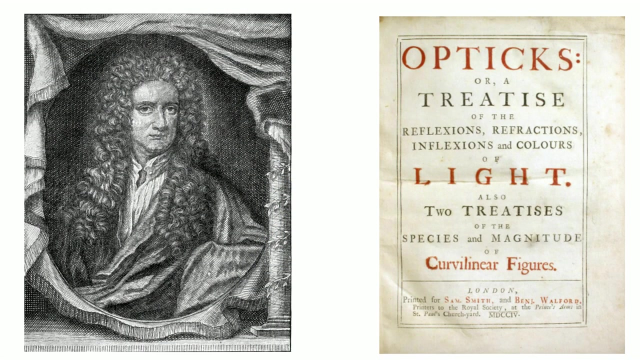 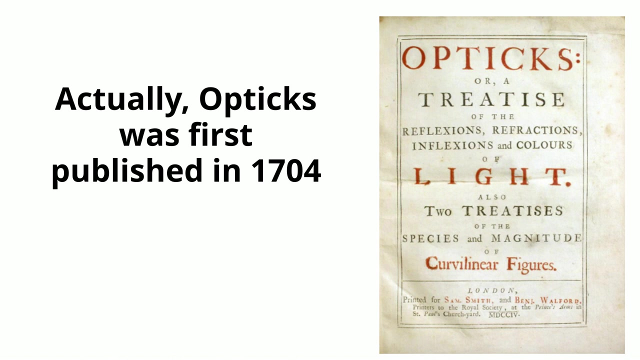 light. White light is made up of different wavelengths, which results in us seeing different colors. If white light passes through a prism, you can see these different colors- Interesting science fact. Sir Isaac Newton described how white light is made up of different colors in 1671 in his book Optics: An easy way to remember the colors of visible light. 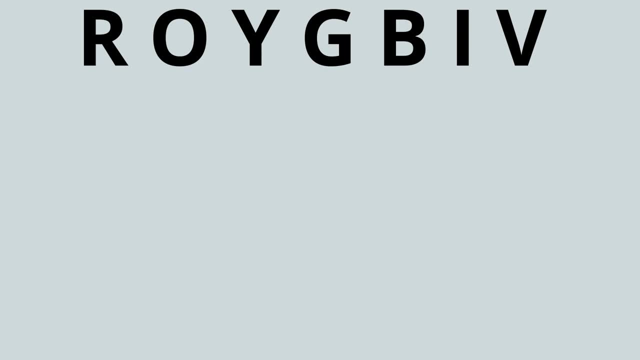 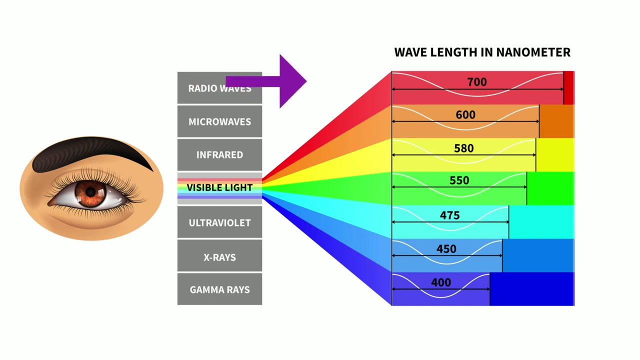 is to use the name ROYGBIV, which stands for Red, Orange, Yellow, Green, Blue, Indigo, Violet, Red light is found at the lower end of the visible spectrum. It has a longer wavelength of about 740 nm. Light in the middle of the spectrum is seen as green and light at the 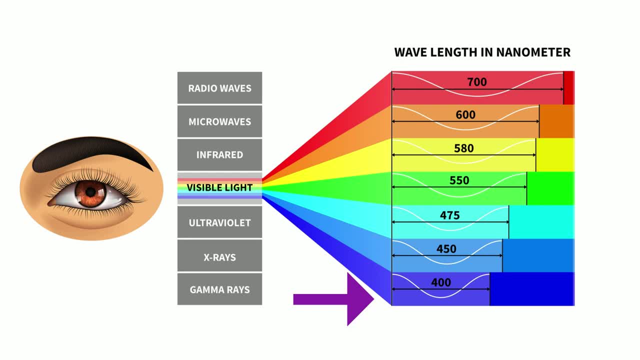 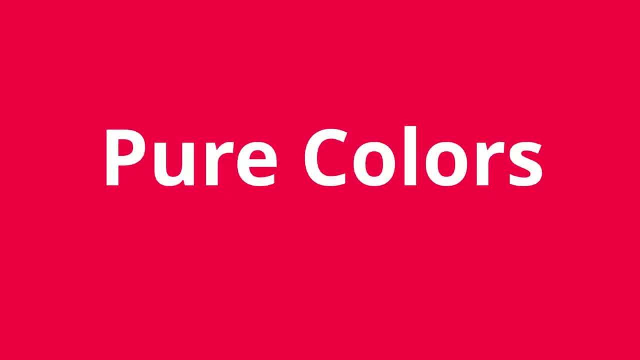 upper end of the spectrum is green, Which has a wavelength of around 380 nm, is seen as violet. Colors containing only one wavelength are also called pure colors, and they are red, green and blue. All other colors that we perceive are mixtures of these colors. Red light has the lowest frequency and photon 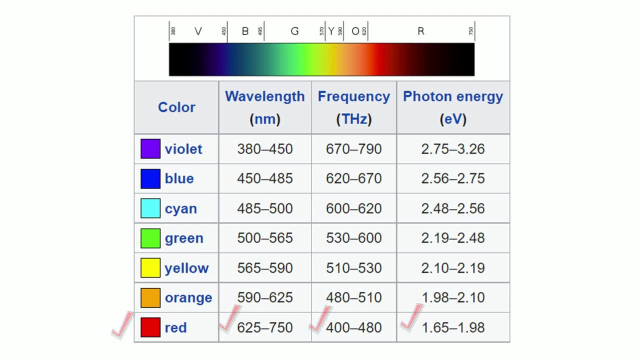 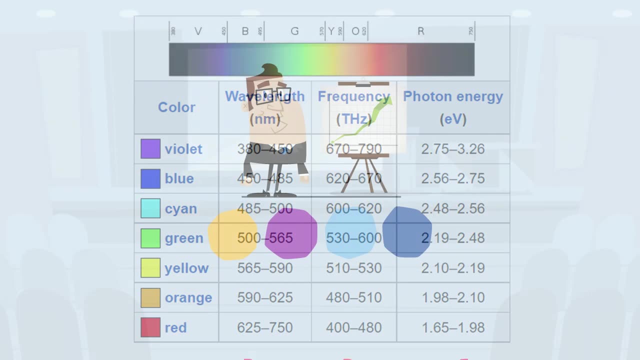 energy, along with the longest wavelength, and violet has the highest frequency and photon energy, along with the shortest wavelength. Here's a nice chart summarizing wavelength, frequency, photon energy and wavelength. Thanks for watching and remember: kindness multiplies kindness.